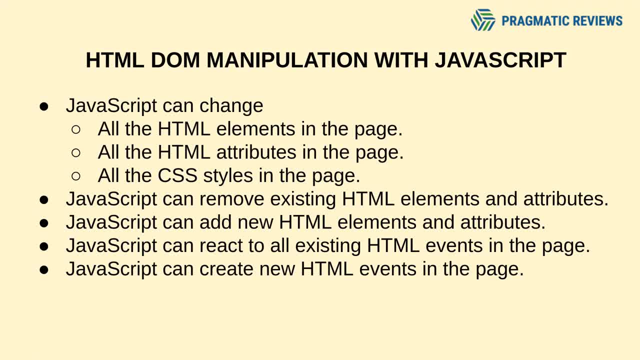 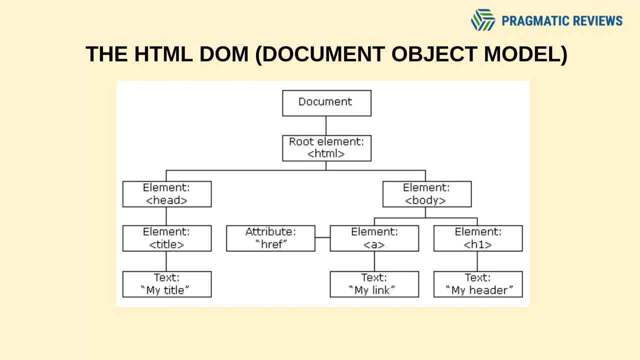 new HTML events within the page. As you may remember, in a previous video on HTML crash course that I uploaded a few days ago, we've been reviewing this document object model, where we have the root element, that is, the HTML tag, and then we have two childs, the head and the body, and then we have some other child for 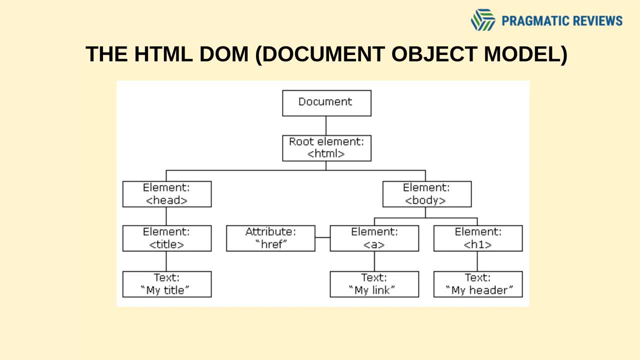 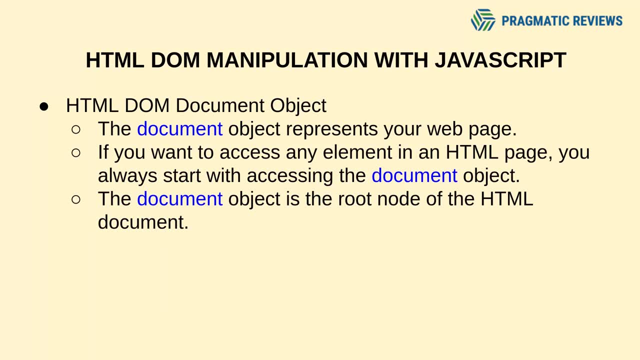 example, the body has the a tag and the h1 as childs. So the HTML DOM document object represents your web page. If you want to access any element within an HTML page, you always start with accessing document object, and the document object is the root node of the HTML document. 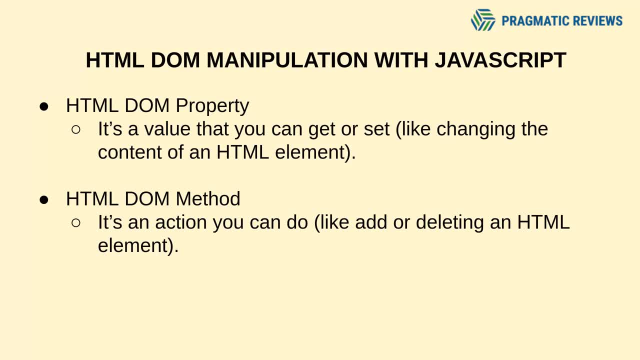 before jumping into the different properties or the most important properties and methods that the HTML DOM API provides in order to manipulate the DOM, let's review what a property and a method are. So. an HTML DOM property? it's a value that you can get or set, that you can read or write, like changing the content of an HTML element. 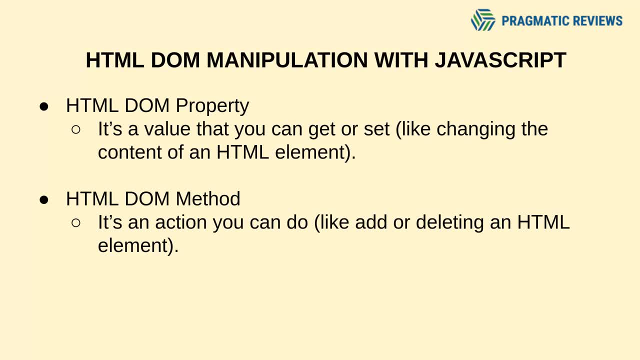 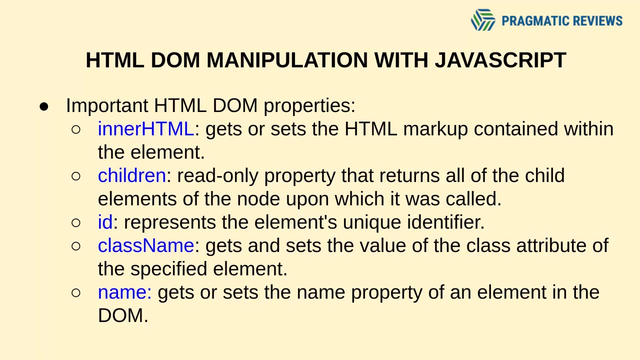 And an HTML DOM method. it's an action that you can do, like adding or deleting an HTML element. Some of the most important HTML DOM properties are: the inner HTML property that gets or sets the HTML markup contained within an element. The children property that returns an array of all the child elements of the node upon which it was called. 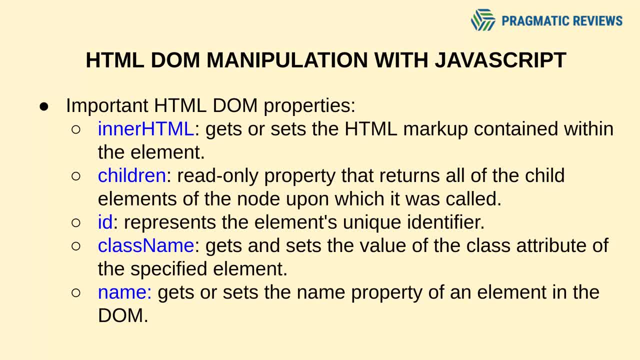 The ID property represents the element's unique identifier And the class name property gets and sets the element's unique identifier. And the class name property gets or sets the value of the class attribute of the specified element. And the name property gets or sets the name property of an element in the DOM. 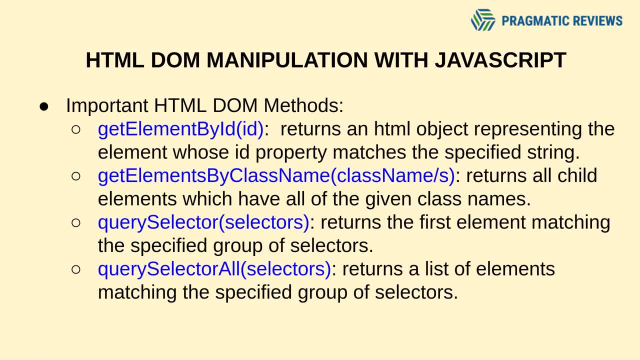 Some of the most important HTML DOM methods are getElementById, getElementsByClassName, querySelector and querySelectorAll. getElementById is a function that returns an element, And it returns an HTML object representing the element whose ID property matches with the specified string. 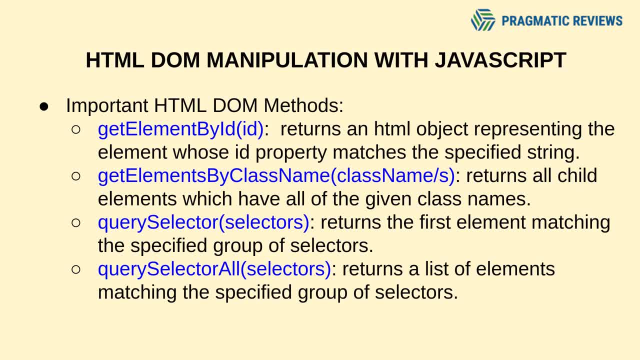 So to this function you pass an ID as an argument, So it's going to return the HTML object that has that value in the ID property. The getElementsByClassName returns all child elements which have all of the given class names You can pass as an argument. 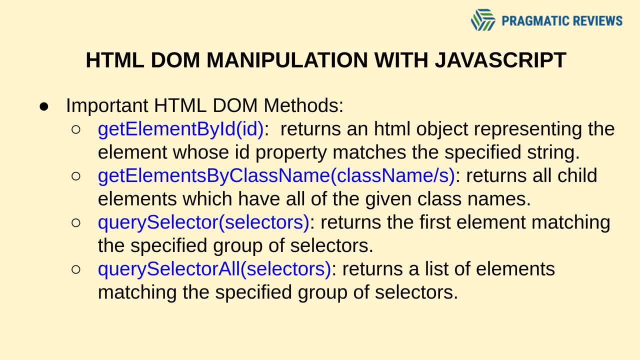 One class name or multiple class names, And then we have the query selector that returns the first element matching the specified group of selectors. We may pass as an argument one or more selectors, And the same happens with the query selectorAll, But in this case it does not return just one element, but a list of elements matching the specified group of selectors. 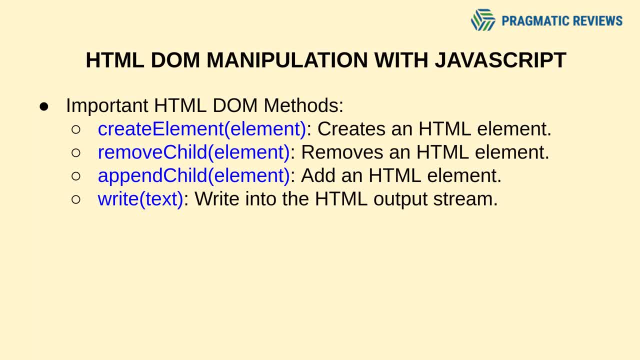 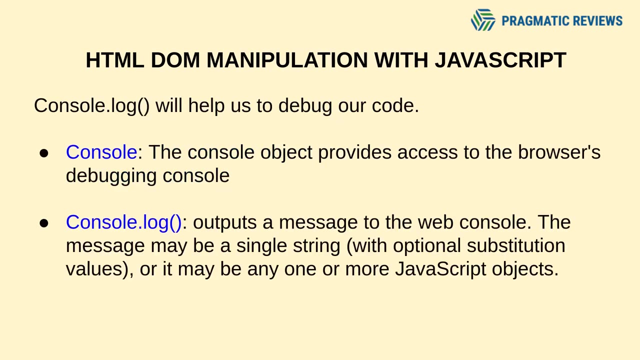 So, more than important, The other HTML DOM methods are: createElement to create a new HTML element, removeChild that removes an HTML element, appendChild that adds a new HTML element, And write that writes into the HTML output string. So, before jumping into the IDE and before start coding on JavaScript and HTML, 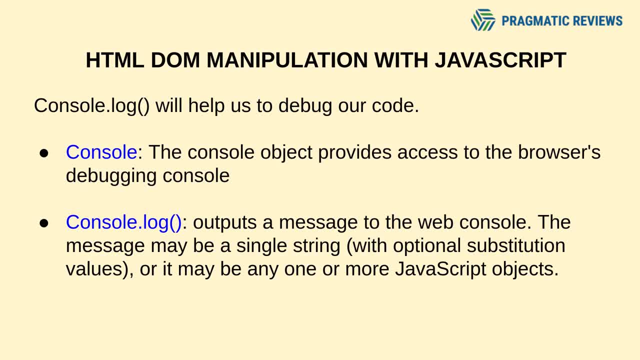 I just wanted to review what the console log is. The console log will allow us to output a message or output different JavaScript objects to validate that the changes that we are doing on the DOM are working. as we expect, We're going to use Chrome, so the console log will output these messages and JavaScript objects in the Chrome's debugging console. 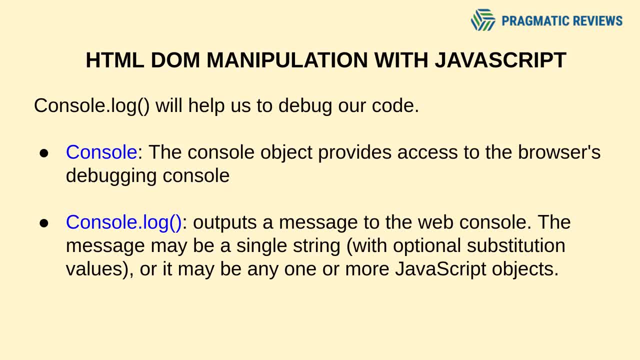 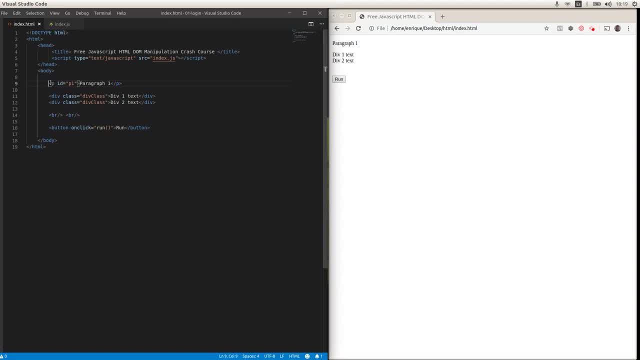 So let's jump to the IDE And let's start coding. OK, we are going to be working on this HTML document. It's pretty basic. It only contains a paragraph, a couple of divs and a button, And here I included a JavaScript file using this script tag, where you need to specify the type that, for JavaScript, is going to be: text forward, slash JavaScript. 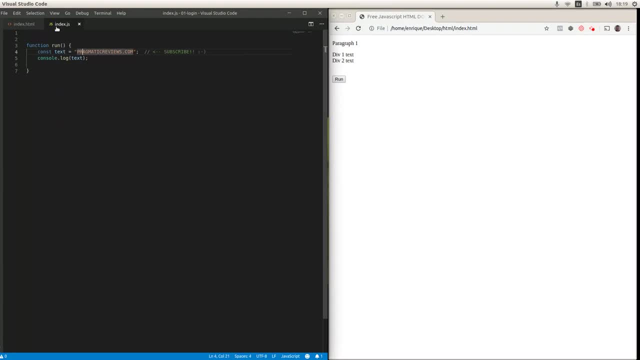 And the source that's going to be the indexjs. that is actually this file. it only contains the run function and is just doing some consolelog of a constant text. that is pragmaticreviewscom. By the way, remember to subscribe to the YouTube channel. 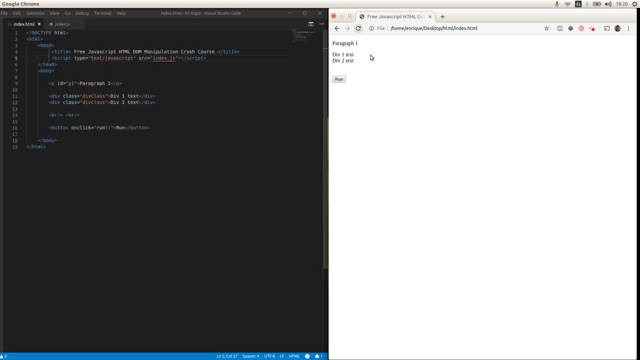 OK. so if we refresh this and we click on run, Let me first open the debugging console of Chrome here. If you click on run, you're going to see pragmaticreviewscom. OK, so let's do something more interesting here and let's change the text within this paragraph. 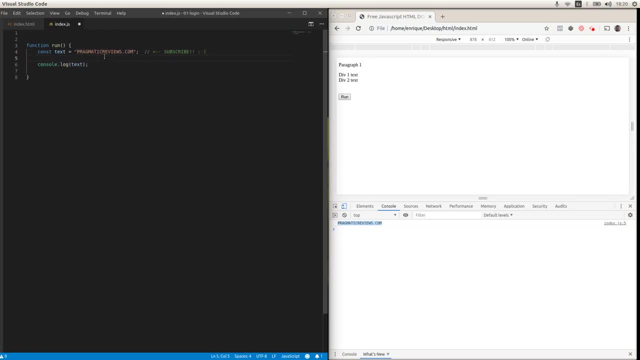 So, in order to do that, I'm going to create a constant. OK, So I'm going to create a constant that's going to be actually the paragraph element. In order to access that paragraph, I'm going to use get element by ID. 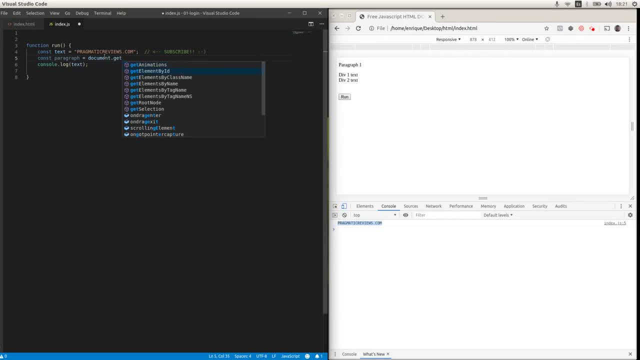 So document that get element by ID, And I'm going to copy and paste the elements identifier, That is P1 in this case. Once we have the element, what I'm going to do is I'm going to change the inner HTML and I'm going to assign a text here. 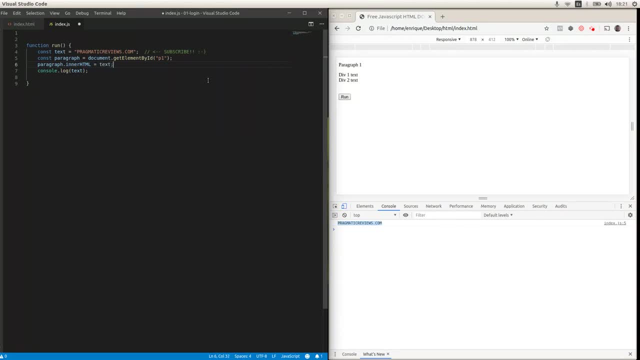 That's going to be pragmaticreviewscom. So let's save this, Let's refresh And let's click on run. OK, So we are still logging the same Value And if we inspect The HTML, We're going to see that the paragraph changed. the text of the paragraph actually changed to pragmaticreviewscom. 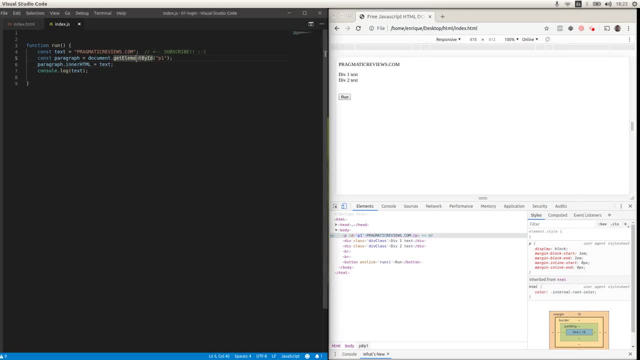 So here we are, using the get element by ID method and the inner HTML property. OK, Now let's Access This list of divs And in order to do that, I'm going to use the. Let me remove this. I'm going to use the get elements by class. 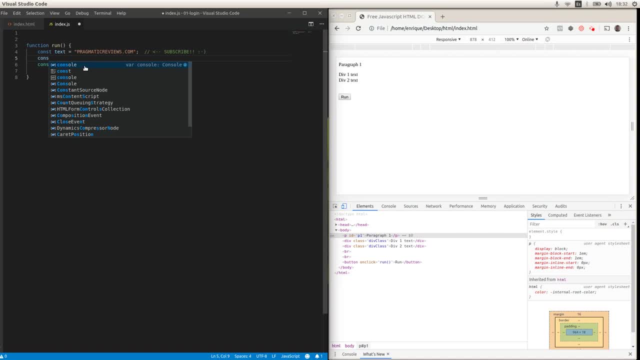 So I'm going to define a constant As divs And I'm going to use document that get elements by class name Actually, And I'm going to copy and paste the class name of these two divs And I'm going to log that array of elements. 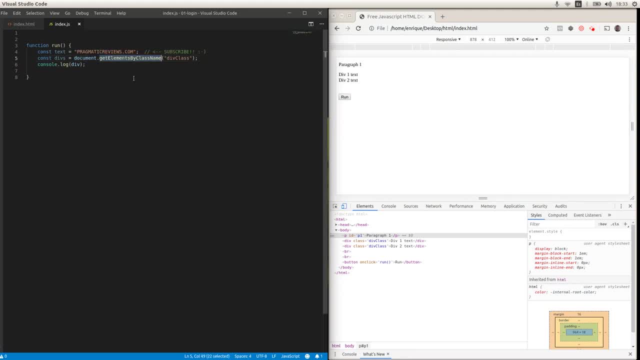 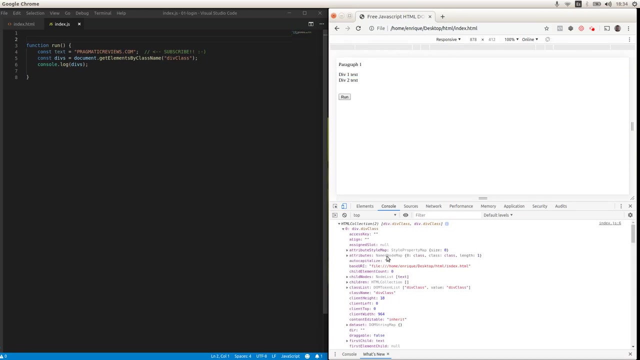 Remember that get elements by class name is going to return an array Of The elements that has div class as the class name. Let's save this again. Refresh, Run OK, And now we have the two elements in the collection. We have the two divs. 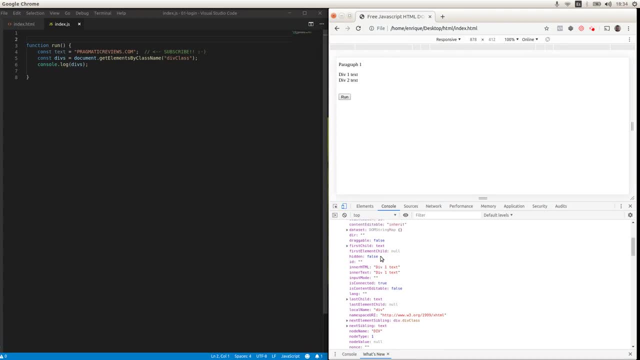 And, as we can see we have, for the first element, we have div one text as the inner HTML And for the second element, That is the second div, We have div two text That are actually what we assign here in the document. 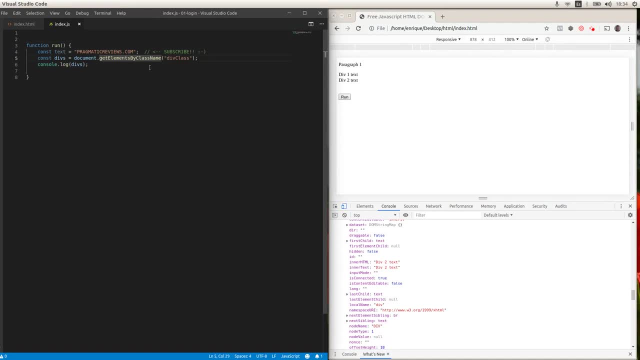 Now let's change the text of the first div. Let's replace div one text by pragmatic reviews dot com. So, as any other collection in JavaScript, we can access the elements By the index in the array. So in this case, the index is zero. 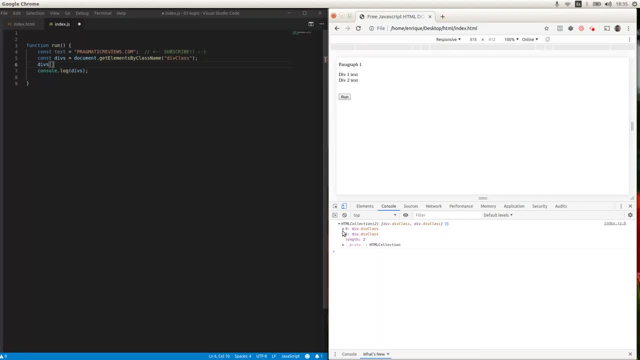 As we can see here on the right in the Chrome's debug console. So I'm going to access that element And I'm going to change the inner HTML property And I'm going to assign pragmatic reviews dot com. That is actually the constant that. 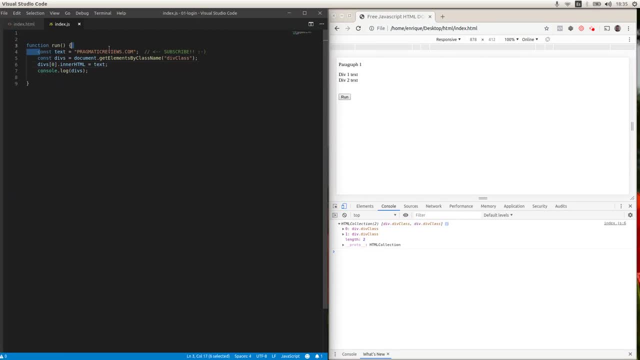 We defined it here at the beginning of the function. OK, I'm going to save, I'm going to refresh And I'm going to click on run And, as you can see here, the text of the first div has been replaced. 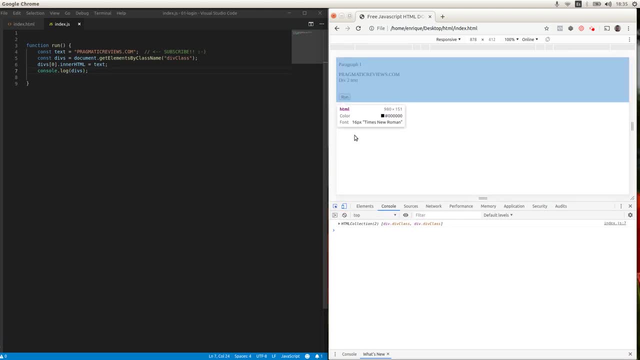 But by pragmatic reviews dot com We can also inspect that div And, as we can see, the text changed to pragmatic reviews dot com. And if you go to the console, we can also see that the inner HTML property changed to pragmatic reviews dot com. 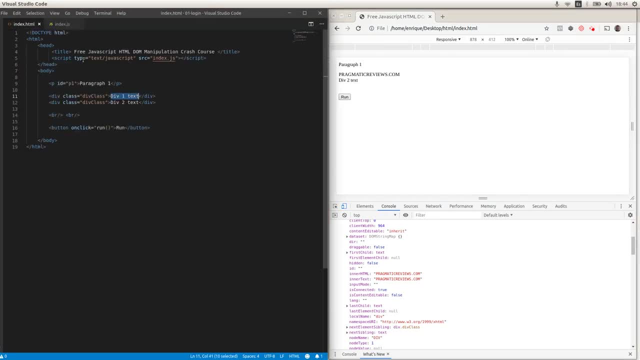 That's what we assign it here. Now, what we are going to do is we are going to append a child to the first div. We're going to append a paragraph within the first div. So let's do some changes here And, in order to add this new paragraph, I'm going to create that node. 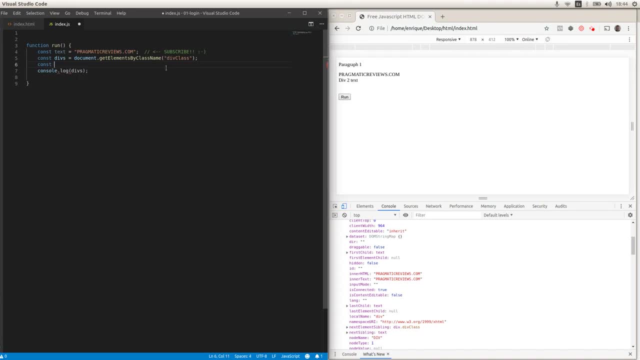 And what I can use to do that is the create element method from the DOM API. So I'm going to create that constant Name it Paragraph And I'm going to do document dot, create element And as an argument I'm going to pass the tag name. 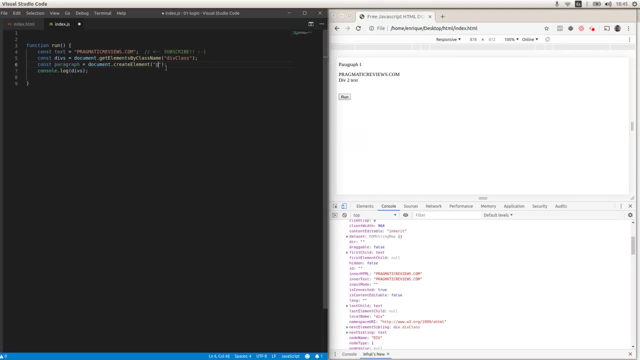 That for a paragraph is the tag p. Now I need to create a text node Just to add some text within the paragraph And I'm going to create a constant named text node And I'm going to create that text node using the create text node method. 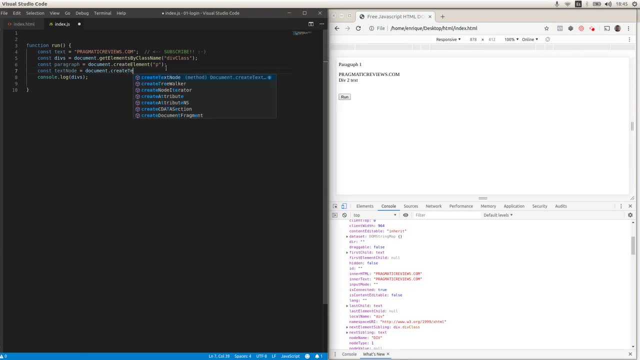 So I'm going to use that one Create text node And I'm going to pass pragmatic reviews dot com As the content of that paragraph. And now I'm going to append the text node to the paragraph. So I'm going to enter paragraph dot- append child. 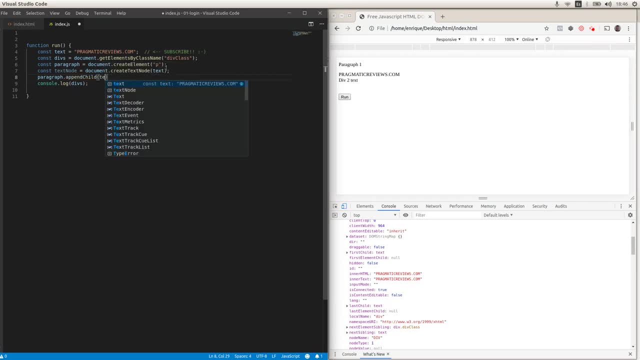 And I'm going to pass the text node as the argument. And now I'm going to grab the first div From the array And I'm going to append the paragraph as the child. I'm going to save this, I'm going to refresh. 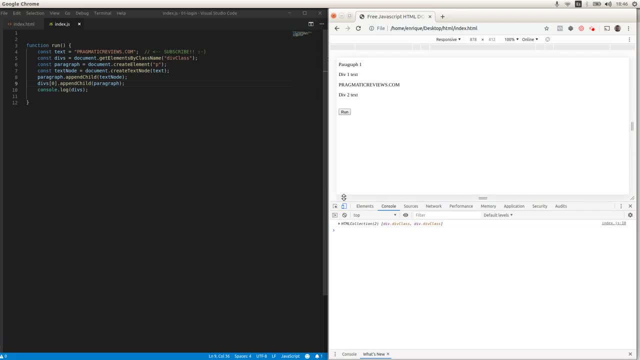 And I'm going to run this function And I'm going to inspect the first div And we're going to see that the div Includes the text that we already assigned to it And also this new paragraph with pragmatic reviews dot com As the text node within it. 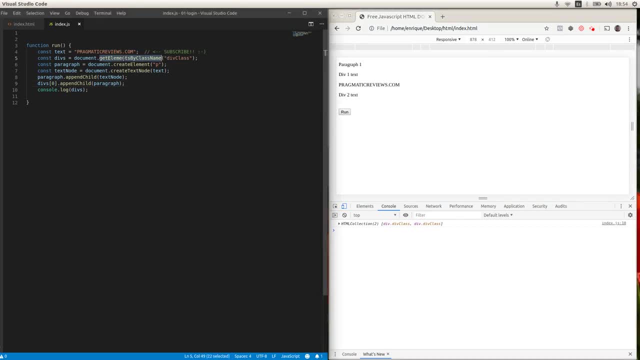 Okay, Now let's make some changes here And let's use query selector all. The result in this case should be the same, Because with query selector all, We also get an array of elements. We need to change the argument, Because in this case, we need to use the selector. 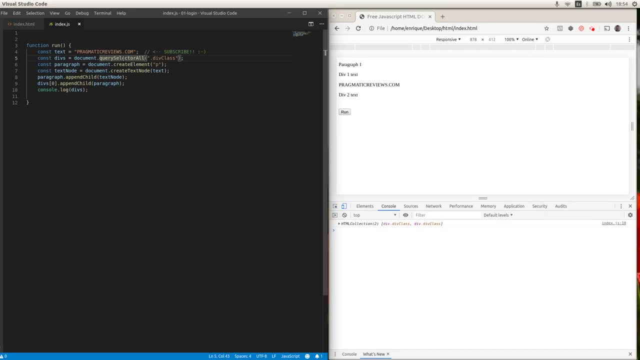 That we use, for example, when we define a CSS selector. So that's why I need to add a period before the class name. So I'm going to save this, I'm going to refresh And we should get the same result. I'm going to inspect the first div. 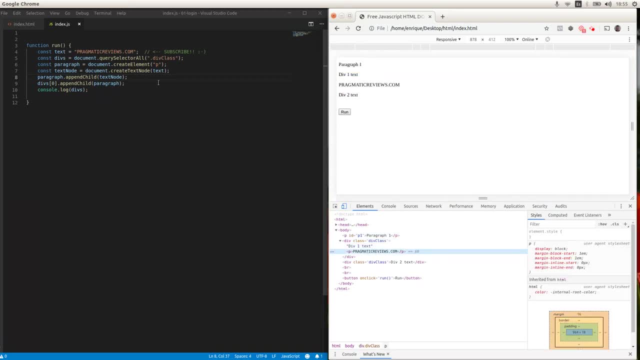 And we have the text And we also have the paragraph that we created here And I'm going to use query selector. The difference between query selector and query selector all Is that query selector returns just one element, The first element that matches with this argument. 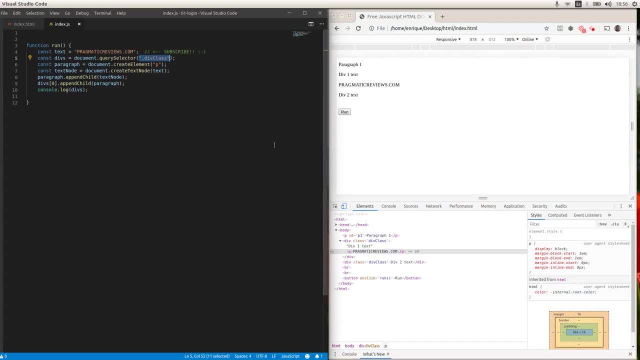 That has the div class As the value of the class attribute And query selector all returns a collection With all the elements that match that argument. So in this case I'm going to rename this constant by div, Because it's going to be a single element. 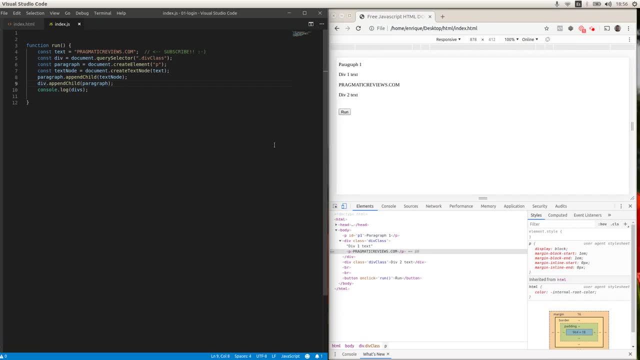 Here I'm going to keep just the div To append the paragraph. And here I'm going to change the log And I'm going to refresh this. I'm going to save this again. I'm going to refresh this. I'm going to run this function. 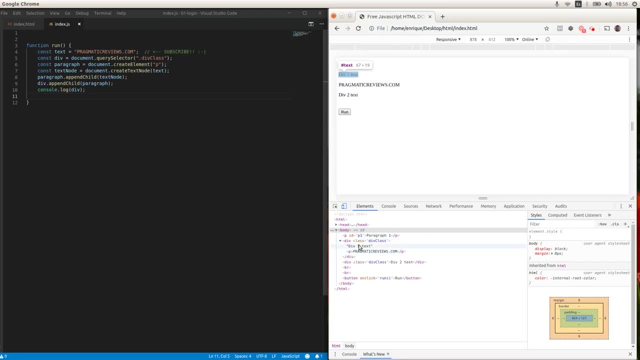 And we should get the same effect. We have the text And we have the paragraph. Let's change the text, Just to validate that what we are doing is actually changing. So I'm going to refresh this, I'm going to run again. 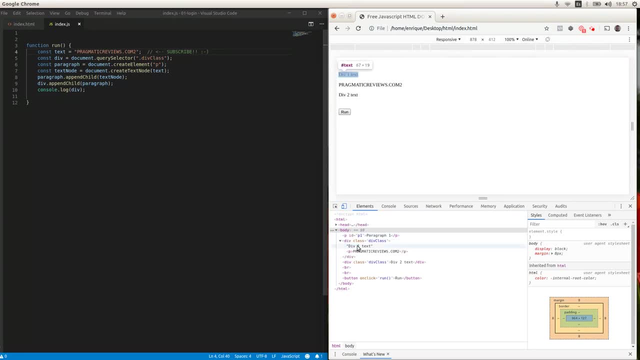 And, as you can see, We have the text that we assigned at the very beginning And we also have the paragraph With the new text that we just changed. Okay, Now, what I'm going to do Is I'm going to use the children property of the div. 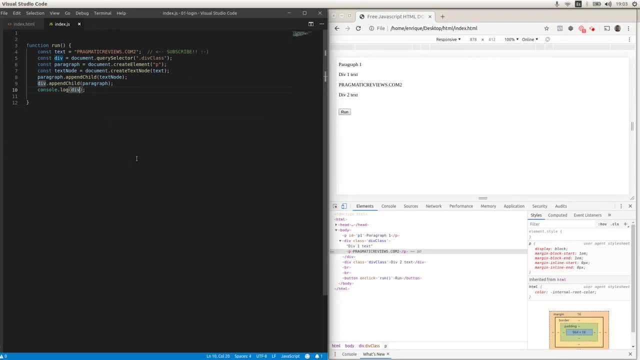 To see that we only have one child. That's going to be this paragraph That includes this text. So I'm going to remove this text Just to be sure that we only have one element as the child. So I'm going to log the children attribute of the div. 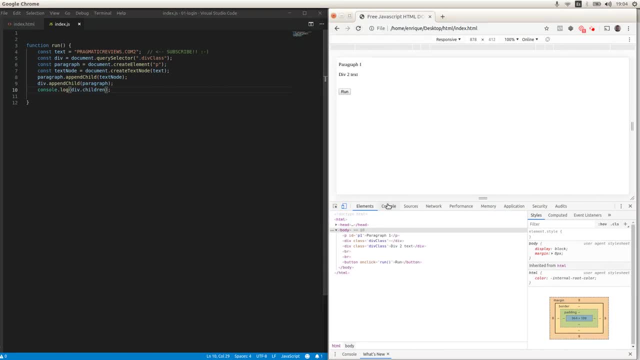 So let's refresh this. Let's go to the console First, run the function And, as we can see, We only have one element, That's the paragraph, And it has the pragmaticreviewscom2 as the inner HTML. Okay, Now I'm going to rename this function. 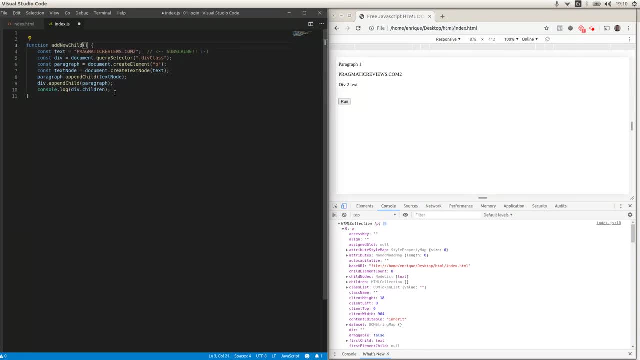 Add new child And I'm going to create a new function And I'm going to name it: Get- remove last child. I'm going to get the div here. I'm going to access the paragraph, So I'm going to create a new constant. 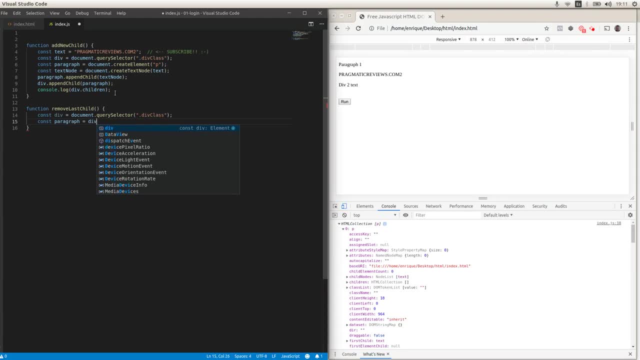 Paragraph equals: div That children, That zero. That's going to be the only element, And this function depends on executing the first one, And what we are going to do is We are going to remove the paragraph By using the remove child. 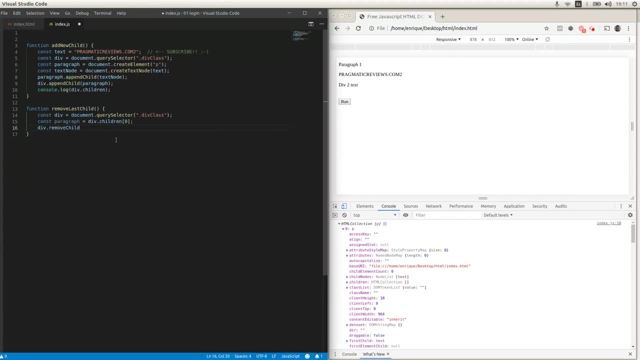 Method And I'm going to pass the paragraph As the argument And we are going to use consolelog To see that I removed The children from the div. Okay, And I'm going to. I'm going to change actually the name of the function here. 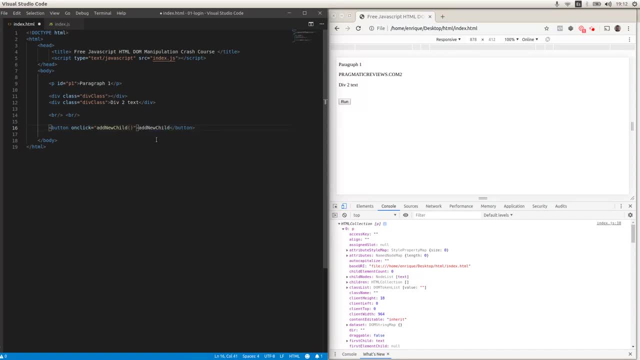 I'm going to change the label of the button Add new child And I'm going to create a new button, Remove last child, And I'm going to invoke from here The new function Named remove last child. I'm going to save this. 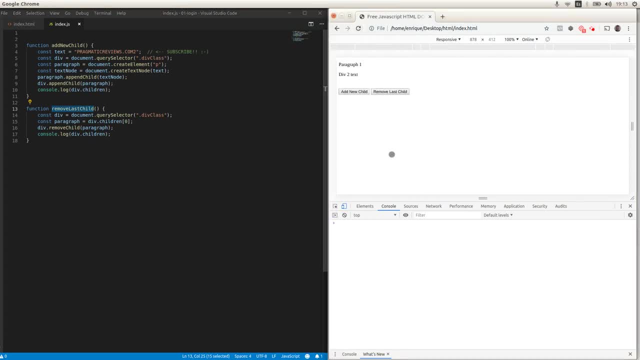 I'm going to save the JavaScript file, I'm going to refresh And I'm going to click on add new child And, as we can see, We have the new paragraph created And I'm going to remove the last child. So if I click on remove last child, 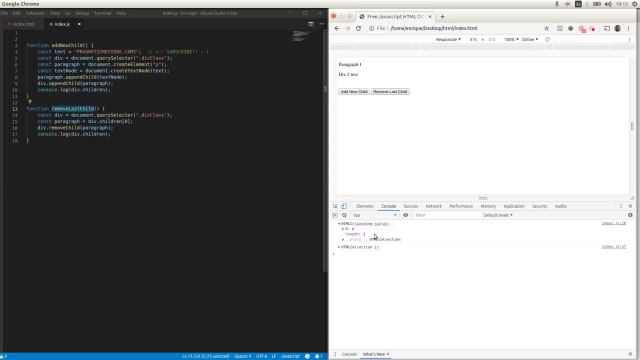 Now I have the children collection empty. I'm going to clear this and execute it again, Just to double check. So I'm going to add a new child. That's going to add the paragraph to the div And I'm going to remove it now. 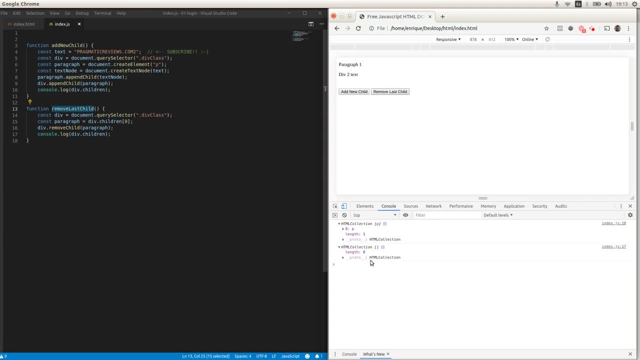 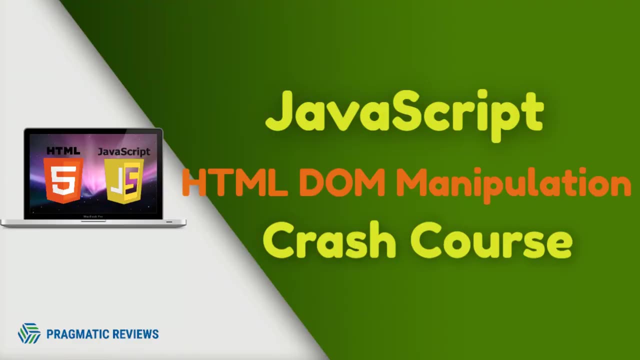 And now we can see that it's no longer a child of the div. Okay, So now you have some of the most important JavaScript and DOM fundamentals In order to be able to modify the contents of your HTML pages dynamically. This is Enrique, with pragmaticreviewscom signing off.